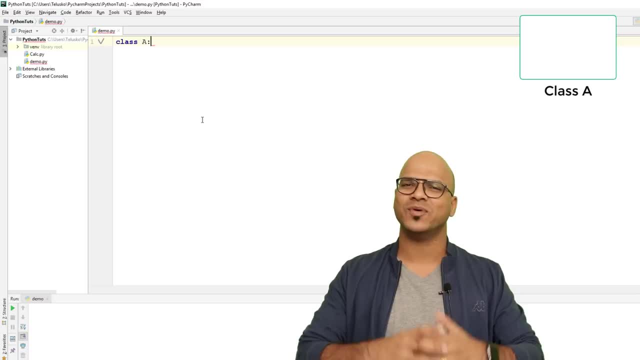 with employee, You can go with student class, You can go with laptop class, whatever class you love, But time being, just for the example, we are going for class A and class B or class C. In future we'll try to implement some other examples using different names and with proper example, But at 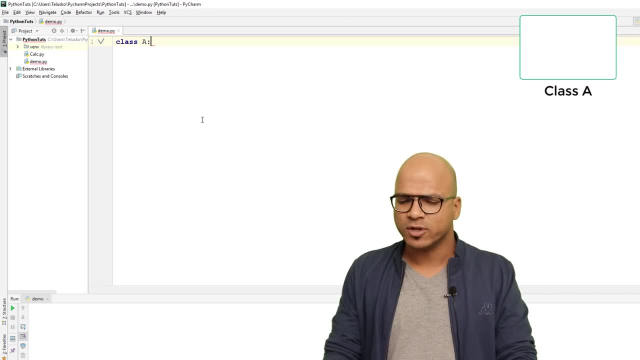 this point. just to keep it simple, let's go for class A. Now, if we talk about this class A, this class A will have multiple features, right? Maybe we can define two methods here, So we'll say: definition there. The first method which I want to go for is, let's say: feature one, okay, So let's. 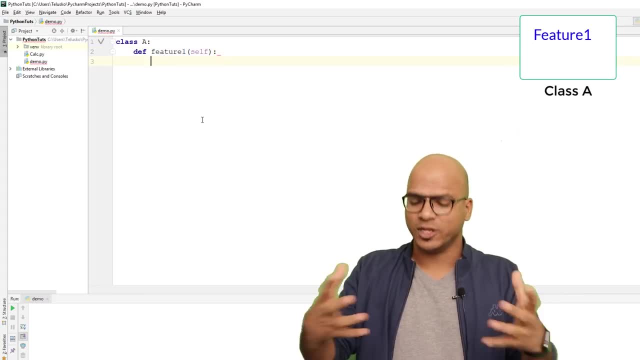 say: we got this function, which is feature one. So let's say we got this function, which is feature one, And this function does provide you something. Okay, So, time being, we are printing feature one working. That's it. Nothing much. Of course it can be a complex code, but make it simple, Let's. 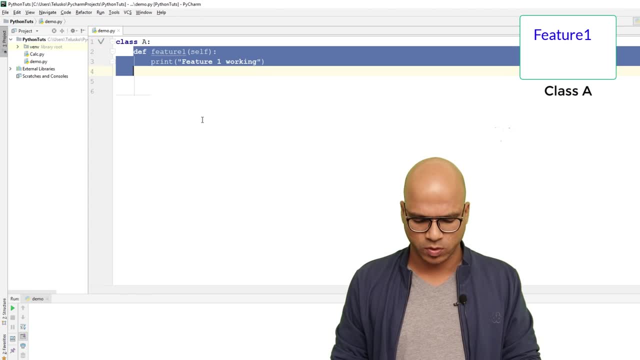 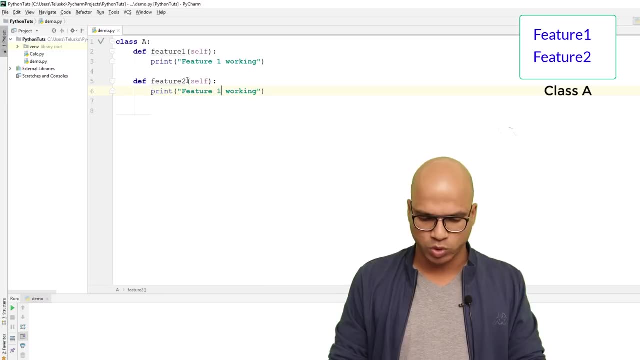 keep it that And then we can have another feature here. Let me just copy paste this code. So I will say copy and paste And this would be my feature two. So we got feature one and feature two And this will print. feature two is working. So this class A has two features. We got feature one. 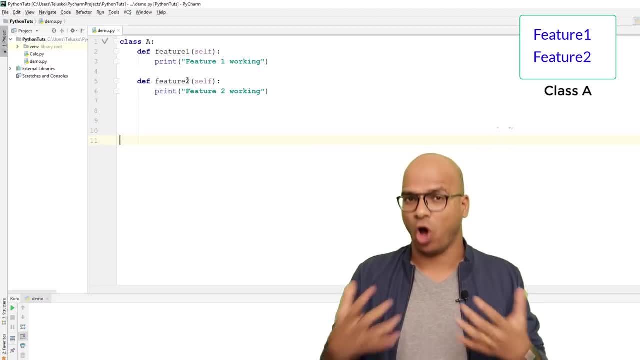 feature two right, And the way you can access them is with the help of object right. And the way you create an object is very simple: You just have to go to the object. You just have to go to the object. For example, you simply say A1 is equal to A. That's how you create the object right. 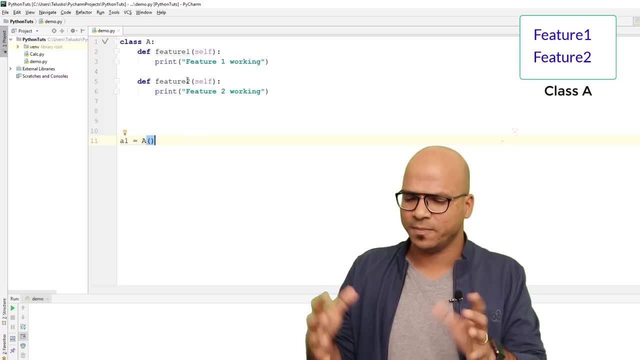 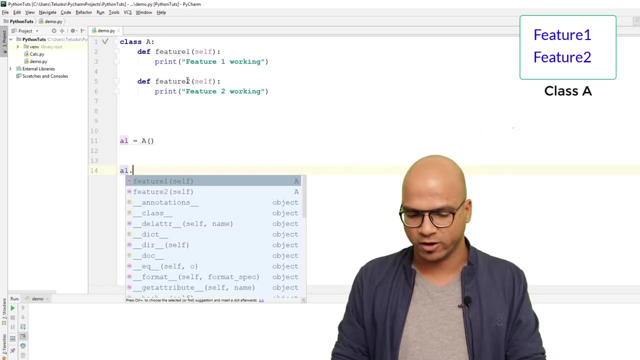 Where A is your constructor. Again, you can find that init method here, but not needed at this point. So this will work. And using this A1, you can call feature one, you can call feature two, right, So you can say A1- dot feature one and A1- dot feature two, And this will work. Let me just 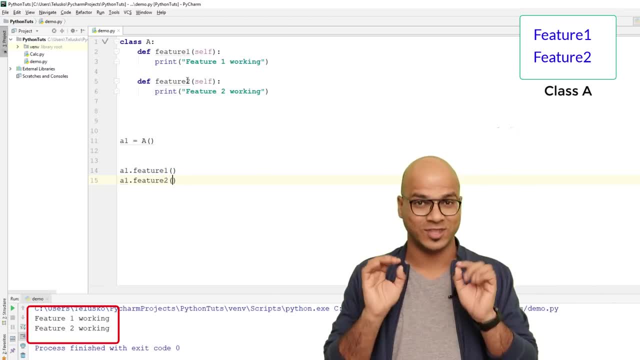 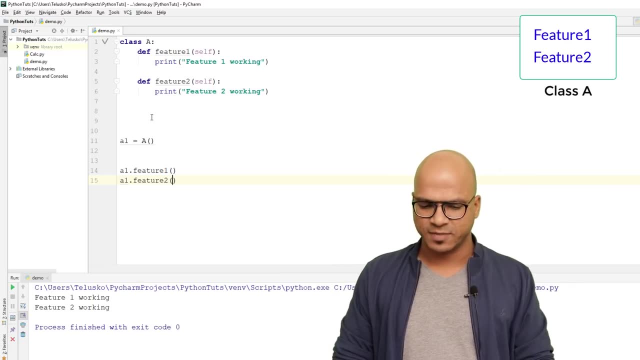 run this code And you can see we got feature one working, feature two working. So this code is working. Now what I'm excited about is, let's say we have one more class, Let's talk about class B. So let me just create a class B here itself. 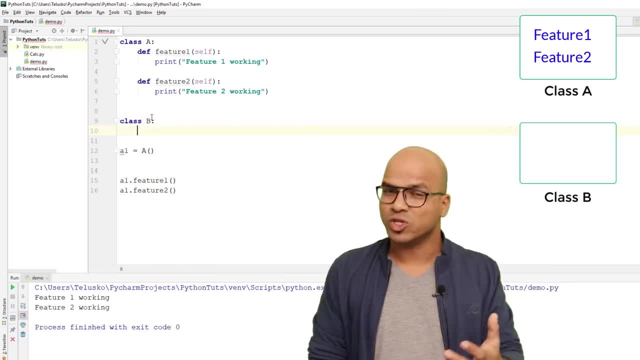 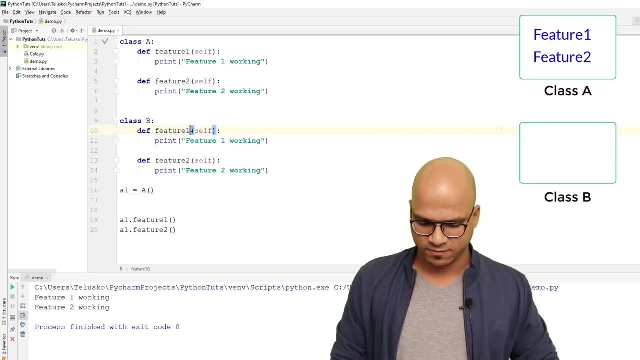 So here I will say class B, And class B will also have two features. I will name this as feature three and feature four. Instead of typing them, let me just copy paste the code here And we'll name this as feature three and feature four. right, See normally what happens, you know. 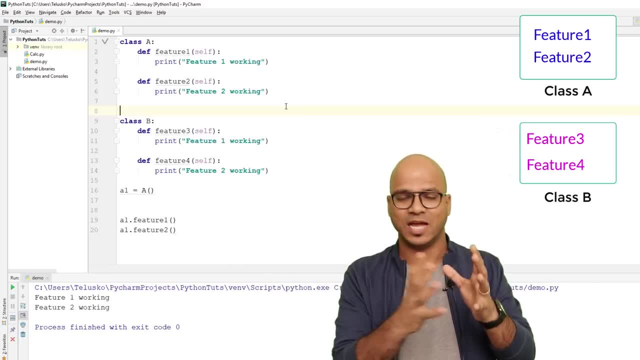 when you work on a project, of course we have a very big team, right? So, example: if one person is defining a class, okay, in that class we provide you four features or four methods. Maybe you want to define some other class in which you need some extra features and you also want the 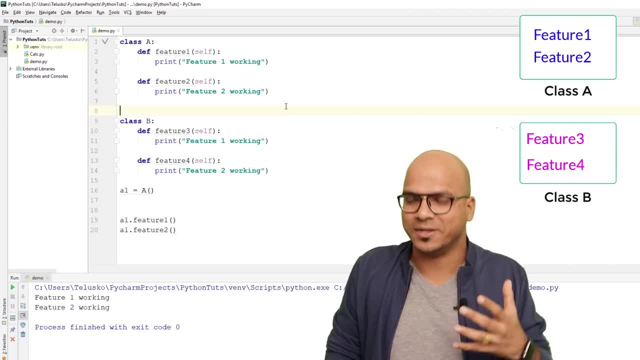 existing features. So let's say you want to define some other class in which you need some extra features. You don't have to redefine it right, You can use it. And the way you do that, you're simply saying: example: in this class B, we got two features, right, We got feature three. 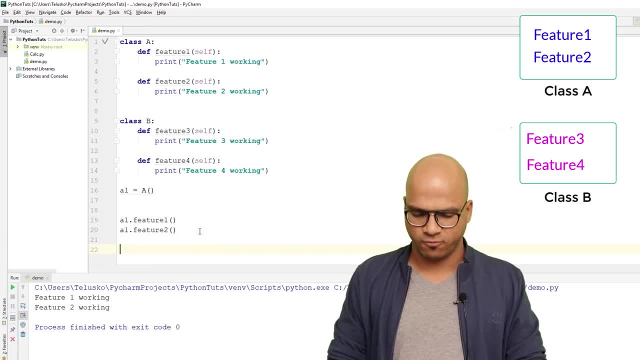 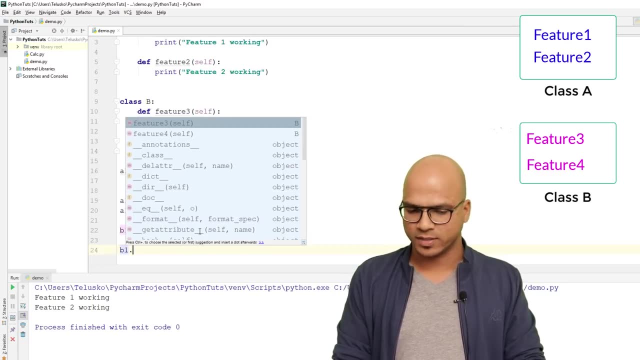 we got feature four And of course, if I create the object of B one, so it's a. B one is equal to B and the functions which you can call using B one. So if I say B one dot, you can see we got. 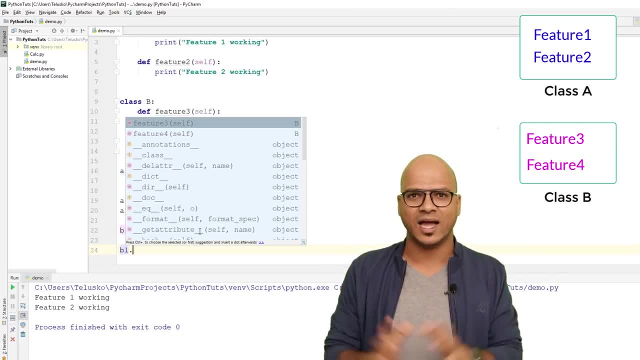 only two options. We got feature three and feature four. of course, right, Because in B class we have only two features. What if you want to get the features of A as well? And that's where the sense comes into picture. So we can say, Hey, this B is a child class of A. right And the moment. 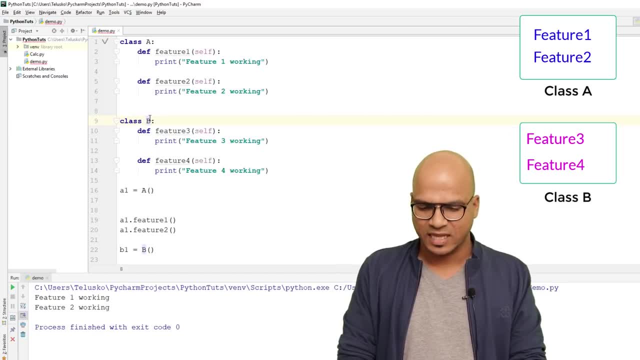 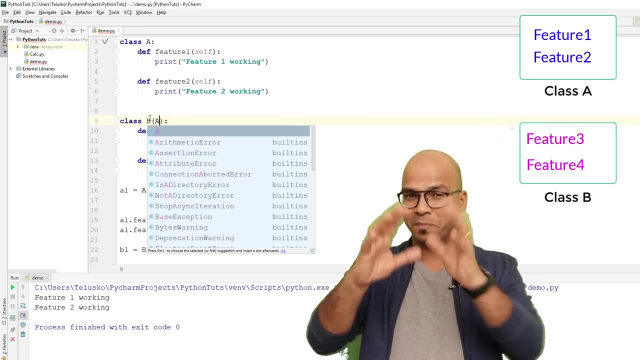 you say child class, it will import all the features. What I will say is this: B is a child class or you can say subclass. We have different terminology we can use here And we can simply say in the bracket you can say A. So this class B is inheriting all the features from A and we got it. 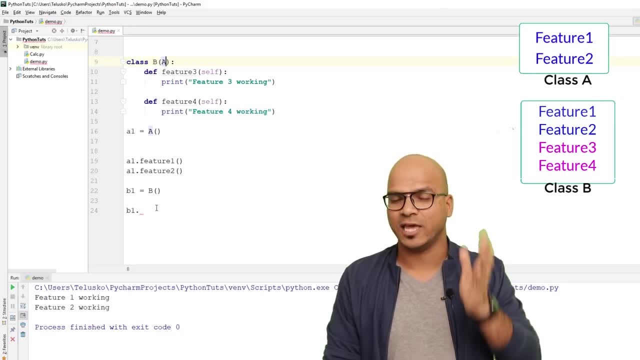 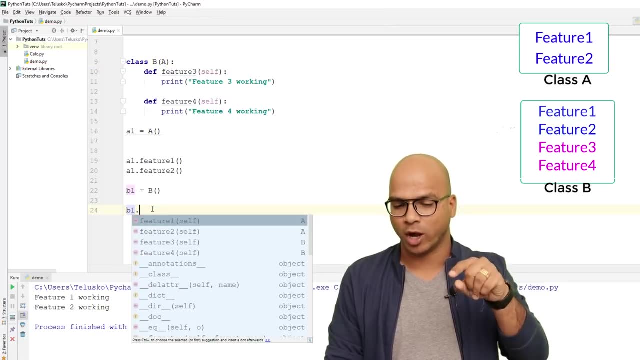 right, Just by adding that one thing, you know, just bracket A, we are saying B is inheriting the features from A, which means With the object of B, which is B one. in this case, the moment I say B one, dot see the options. 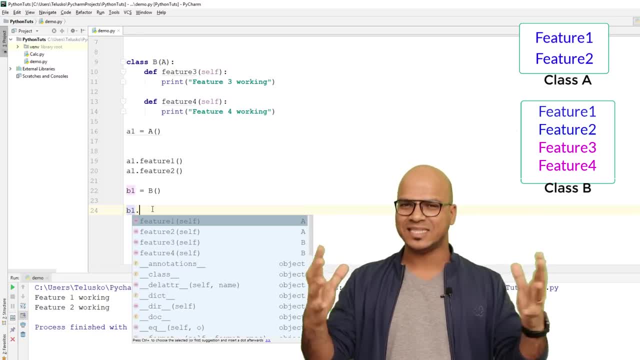 you can access feature one, feature two, feature three and feature four. And that's the importance of inheritance, which simply means if you already have a class which provides you some feature and in future if you want to create your own classes in which you want to use those features. 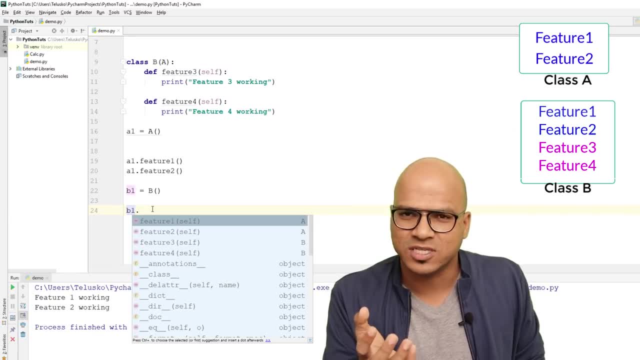 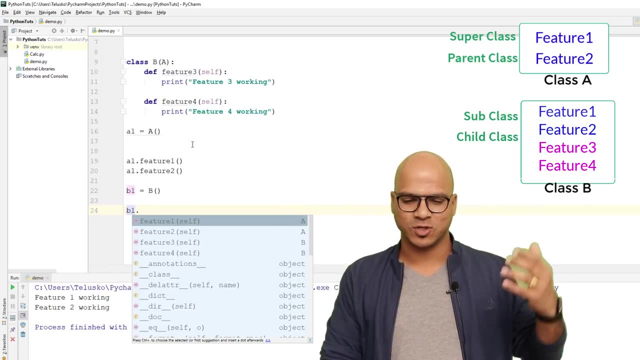 you just need to inherit them, right? So we can use some terminologies here. We can say superclass, subclass, or we can say parent class or child class. So time will refer them as superclass, and super is a class which is A and a class which inherits the class. we will call them as subclass. 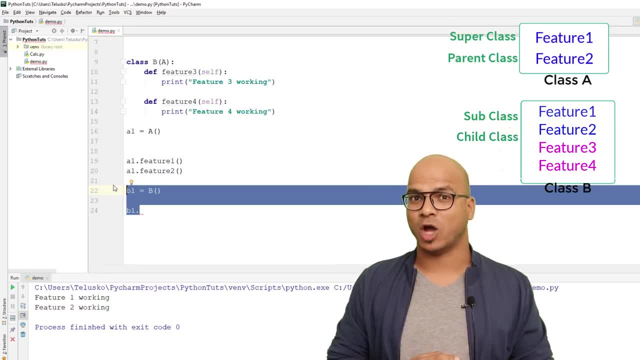 So B is subclass and A is superclass. So that's the concept about inheritance. Now, this is also called as a single level inheritance. We have some other types as well. We also have a multi-level inheritance. Now what it means. example: let's say: if I have another class here, let me get one more. 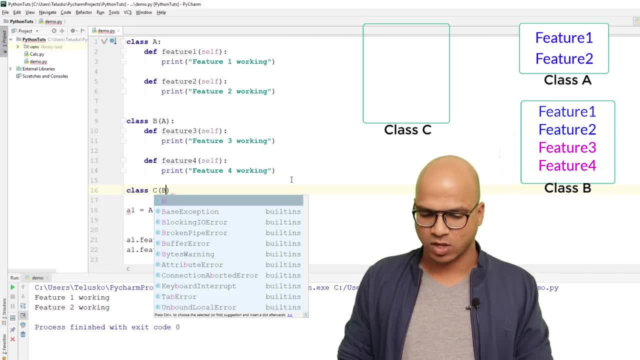 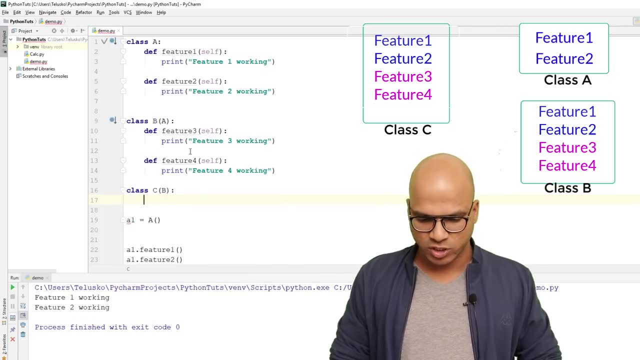 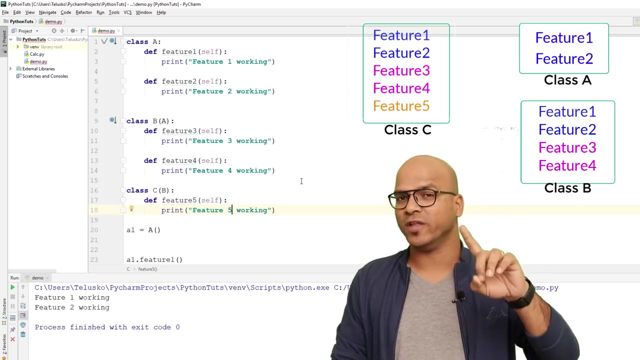 class here and this class is, let's say, C, So we'll call this class C or this class C inherits B. Now this class, let's say time bin. I will define only one feature here. We'll say feature five. You can see how lazy I am. So this is feature five working right. So we got C class, which has only 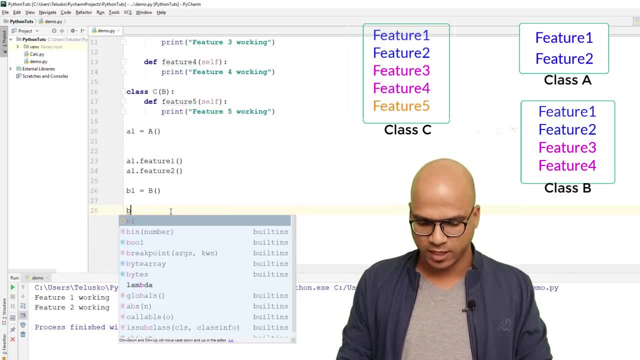 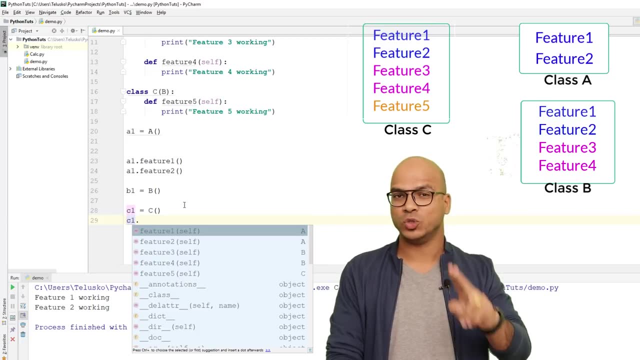 one feature. But the moment you create an object for C1, so I will say C1 is equal to C. The moment I say C1 dot. see the methods you can use. So we can use feature one. Now feature one. feature two: 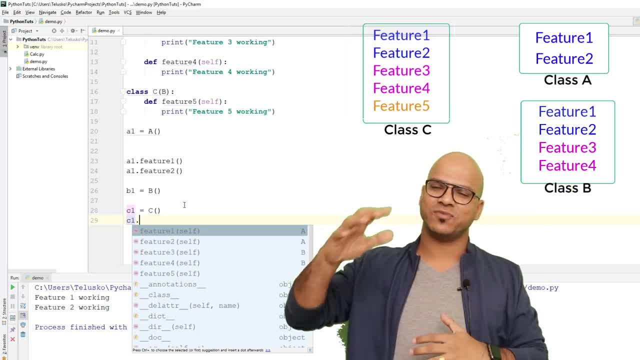 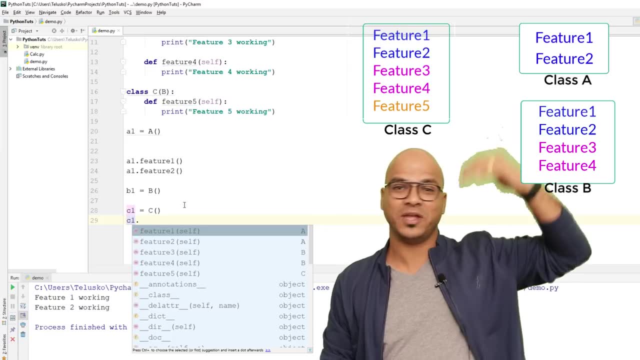 are coming from A right, But C is only extending B. So that's a relationship: We have grandparent, we have parent, and then we have child, right. So a child can access all the features from parent, grandparent, great-grandparent, right. So that's how it works. Okay, this is working right. So 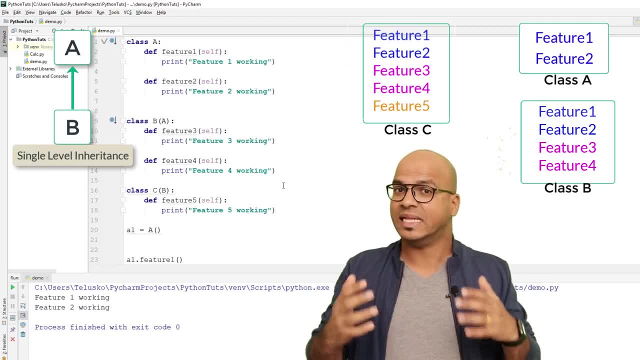 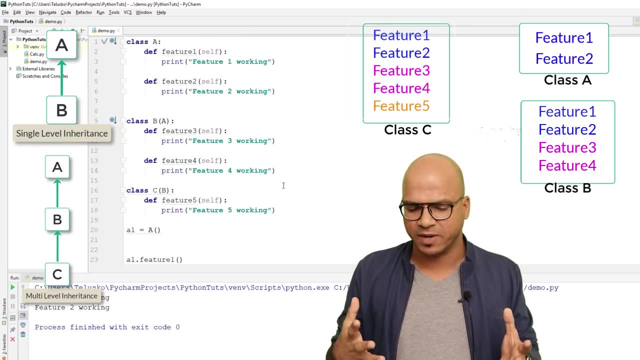 we got single, where you have one superclass, one subclass. then we have multi-level, where you have superclass, subclass and then, I guess, subclass of that superclass. Okay, This is working. What if you go for multiple? What is multiple here? Let's say, the C is not only taking from A and B. 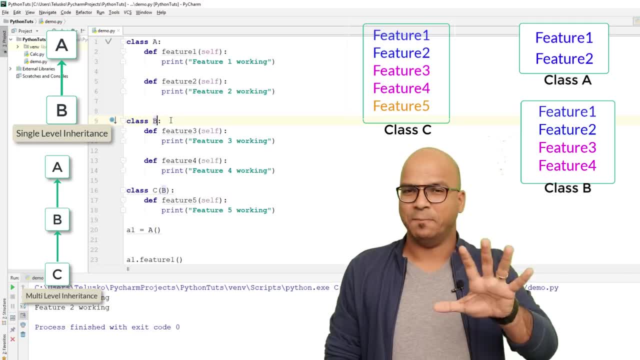 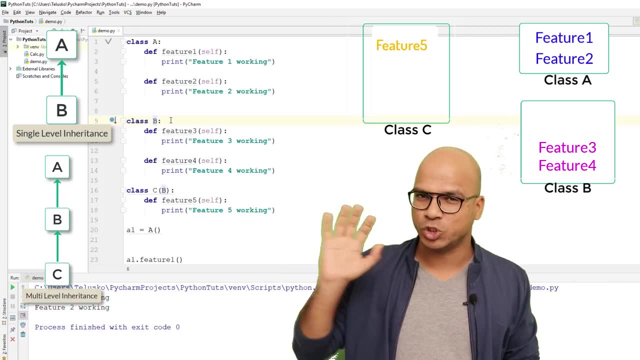 we've got some other class as well, Just for time bin. what I will do is I will say: B is not inheriting A. okay, So A and B they are two different classes. Nothing, they are not related to each other. A provides two features, B provide two features. So let's say B is not inheriting A. 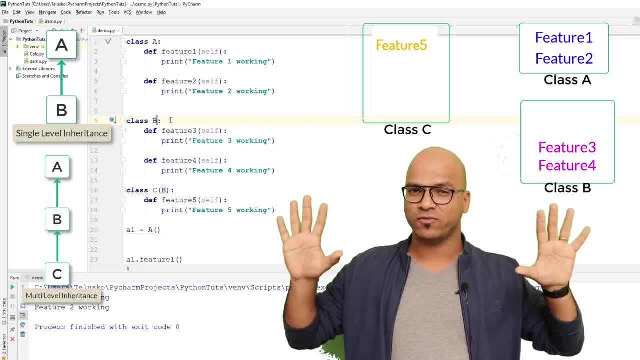 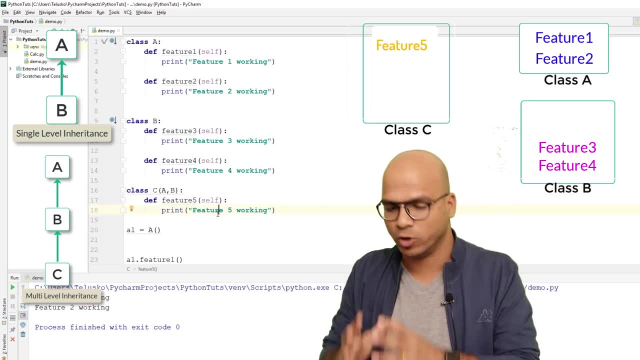 okay, So A and B, they are two different classes. nothing, they're not related to each other. A provides features- okay, so there's no relationship between a and b. there are two different classes. c says: i want to access features from both, from a and b. so in this case, so c will inherit from a and b- both. 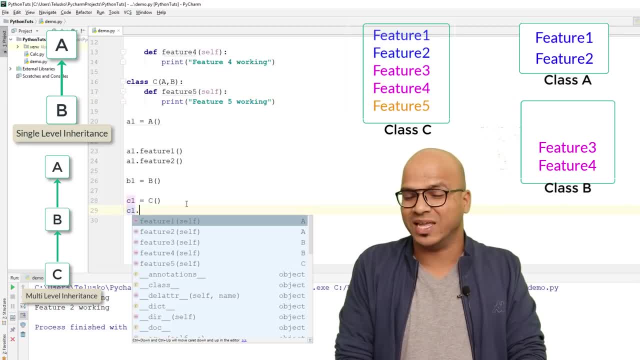 so you will say a comma b, so c will copy from both, or c will inherit from both, so it will say c1. the moment you say c1, you can see you can access all the features. that's not the case with b1. now b1. 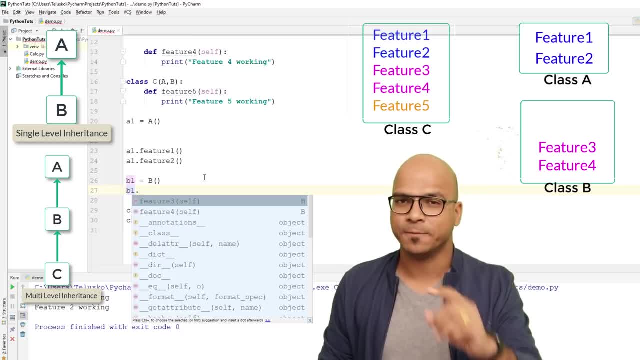 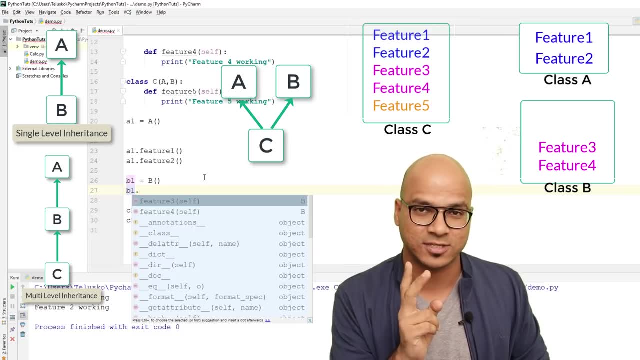 can only access two features, feature 3 and feature 4, because b is not inheriting a. okay point, remember. so we got a, we got b and then we got c. c is inheriting both the classes a and b, so this is called as multiple. so this is your multiple right. so we have done with single, we have done. 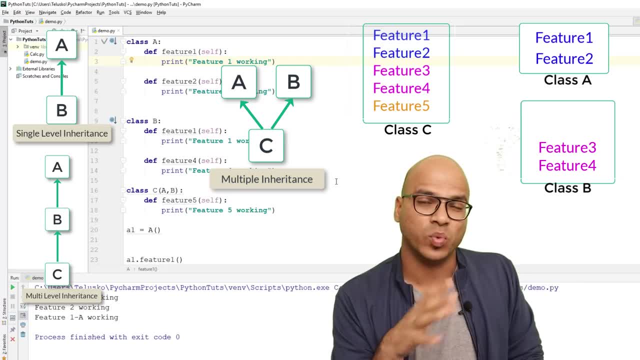 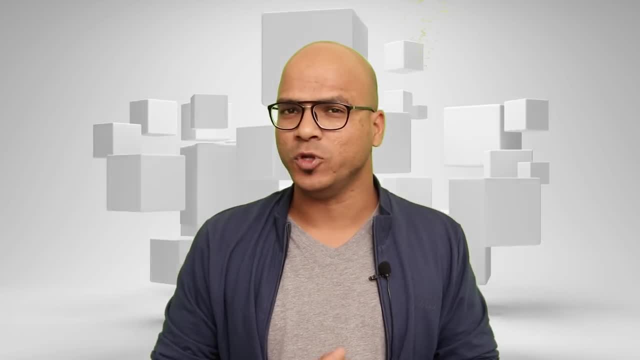 with multi-level and then we have multiple. so this is how we can work with inheritance. in the next video, we'll try to focus more on inheritance and let's see what else we can do with it. so i hope you are enjoying this session. let me know in the comment section and do subscribe for further videos.